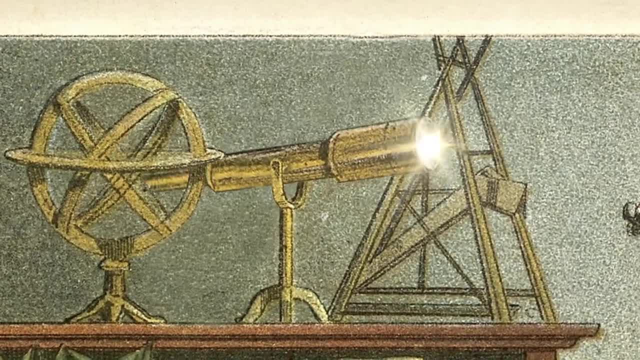 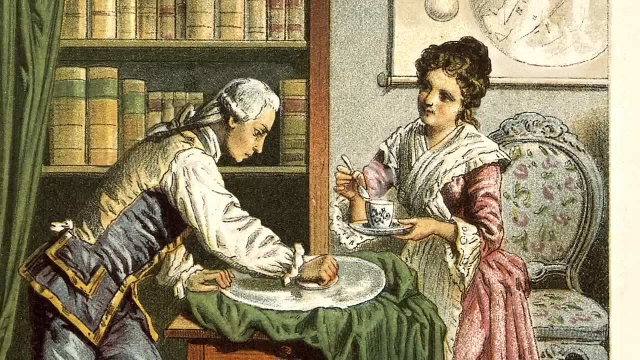 With it, he was able to view the heavens with great clarity. Herschel, with the assistance of his sister Caroline, undertook a survey of the night sky, paying special attention to double stars. On March 13th 1781, Herschel took a closer look. 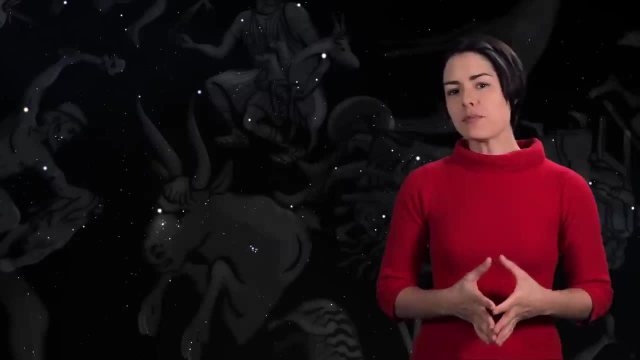 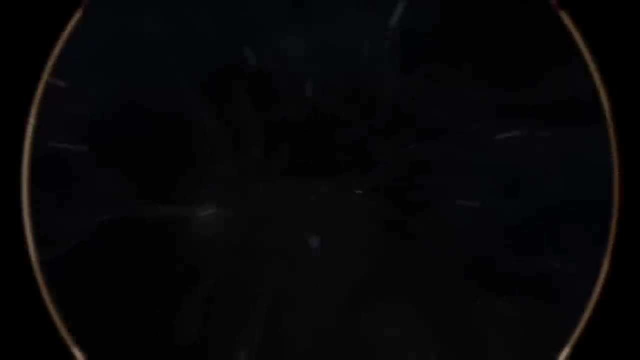 at what was to come. It was assumed to be a faint star. It had been previously catalogued by other astronomers as 34 Tauri, the 34th star of Taurus the bull. Through his powerful telescope, however, Herschel observed it with fresh eyes. 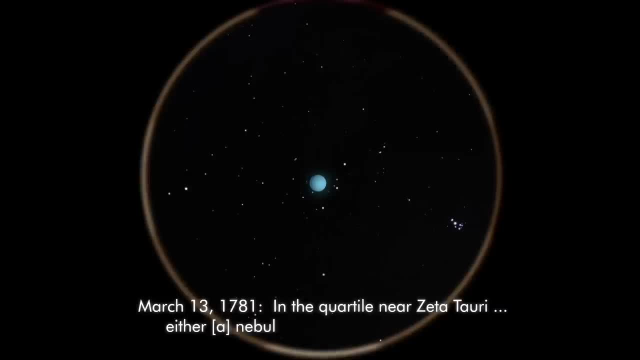 In his notes he wrote: In the quartile near Zeta Tauri, either a nebulous star or perhaps a comet. Four days later, on March 17th 1781, he wrote: I looked for the comet or nebulous star and found that it is a comet. 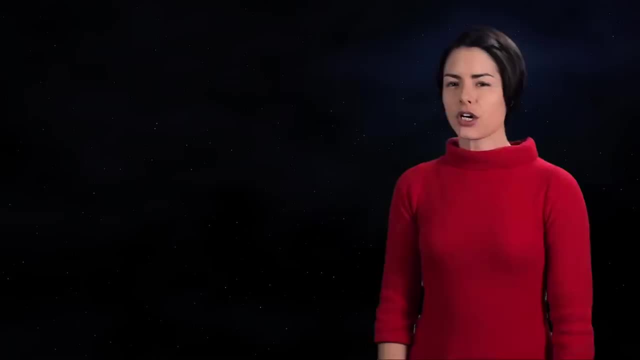 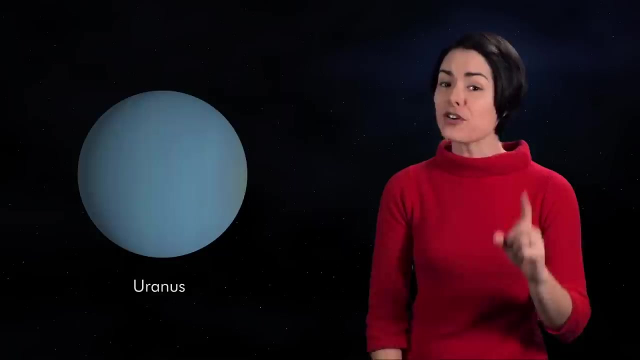 for it has changed its place. Herschel had discovered a new heavenly body that moved. It turned out not to be a comet, but a planet, the first to be discovered since prehistoric times. It was twice as far away from the Sun as Saturn. 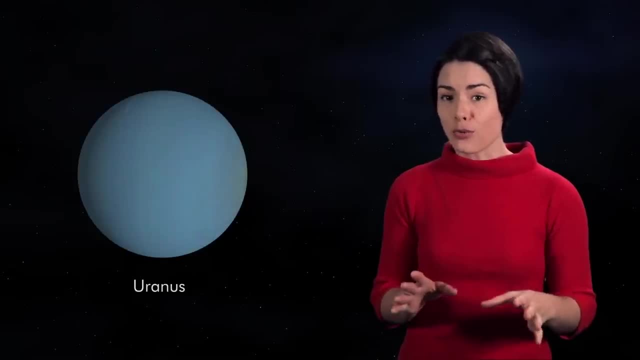 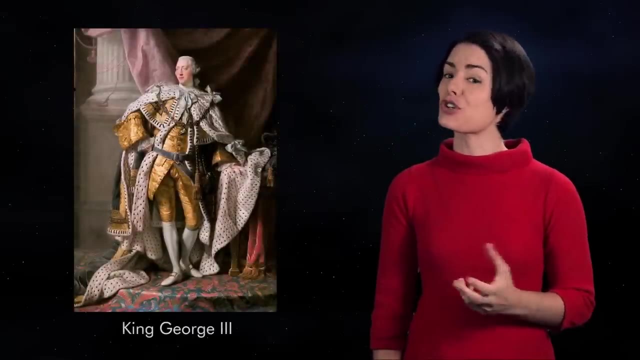 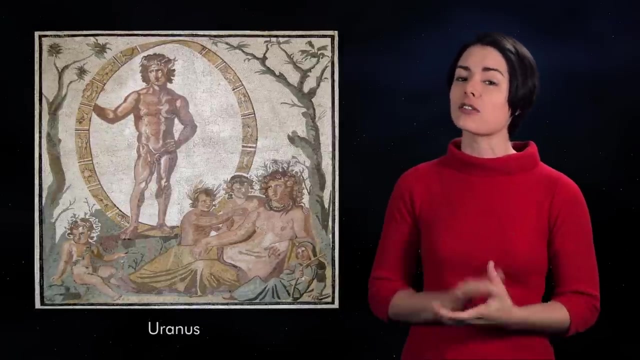 Overnight, Herschel had doubled the size of the known solar system. Herschel wanted to name his find Georgium Situs Latin for Georgian star, after King George III of England. Cooler heads prevailed and the name Uranus was settled upon. which followed the tradition of naming planets after Greek and Roman gods. Uranus was the Greek god of the sky. As news of his discovery spread, Herschel became famous overnight and he was appointed by George III as a royal astronomer. He was elected a Fellow of the Royal Society. 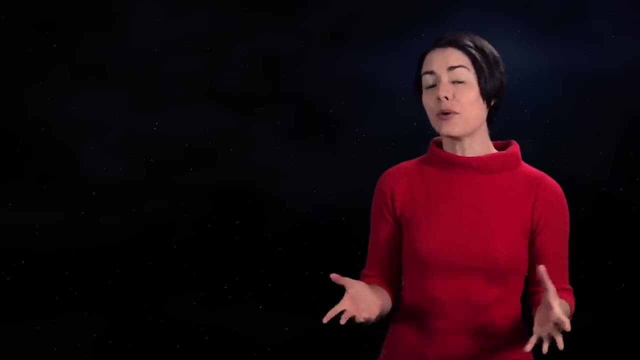 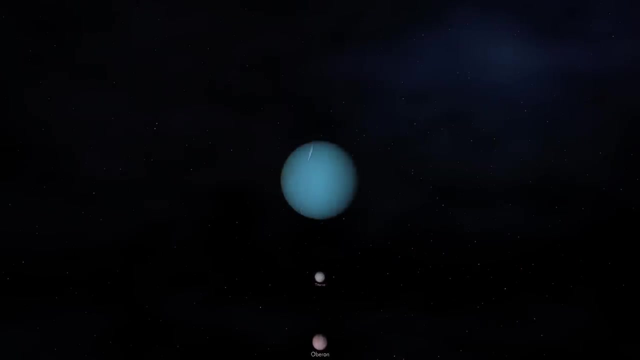 and was awarded grants to continue his work and build more telescopes. Herschel went on to discover two of the moons orbiting Uranus. His son, John, named them Oberon and Titania, after the king and queen of the fairies in William Shakespeare's A Midsummer Night's Dream. Most of the moons of Uranus discovered later were also named after Shakespearean characters: Juliet, Miranda, etc. Herschel was knighted in 1816 for his invaluable contributions to science. His discovery of Uranus shattered the notion that the ancients 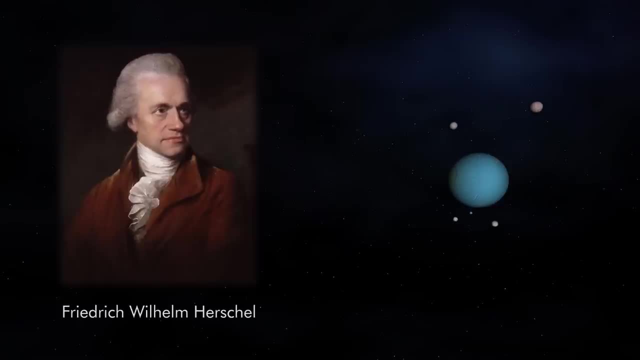 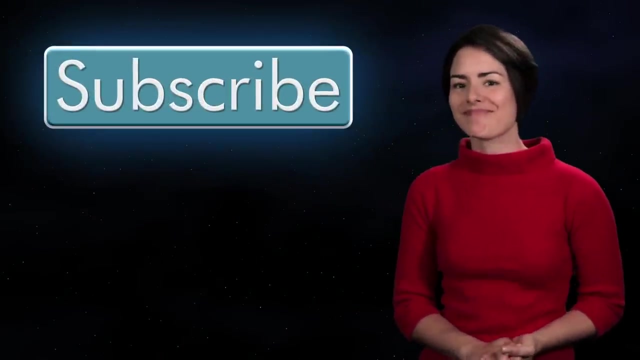 had discovered everything in the solar system. Herschel's work ushered in a new era of astronomy, one in which momentous discoveries were still possible. The universe is a pretty big place, and so is that subscribe button. I'm not going to tell you to click it, because I'm certain you'll do the right thing. The right thing is to click the button.